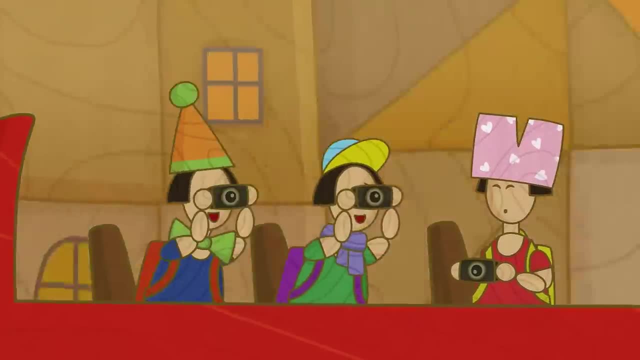 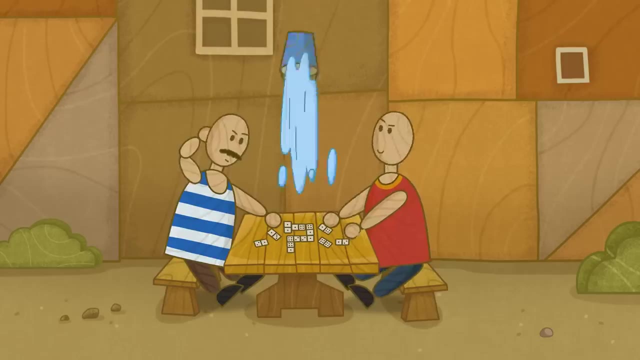 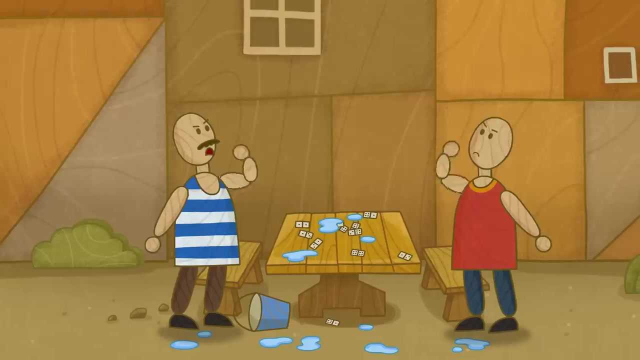 The bus drives along a Companion Street. He is on the way to the bus. If he gets lost, he will be returned to the city as soon as the bus comes. A city bus drives along a Companion Street. He drives around the bus every day. 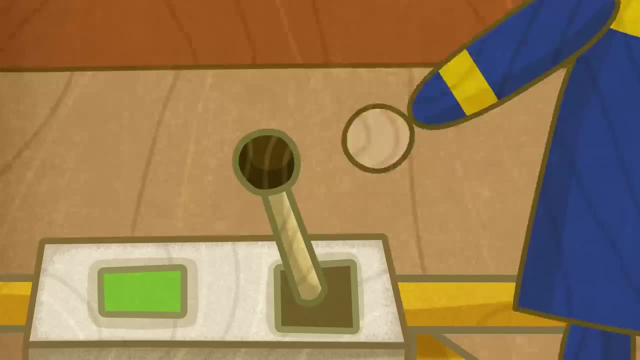 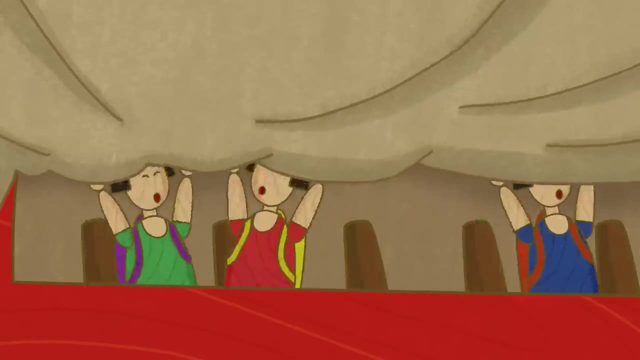 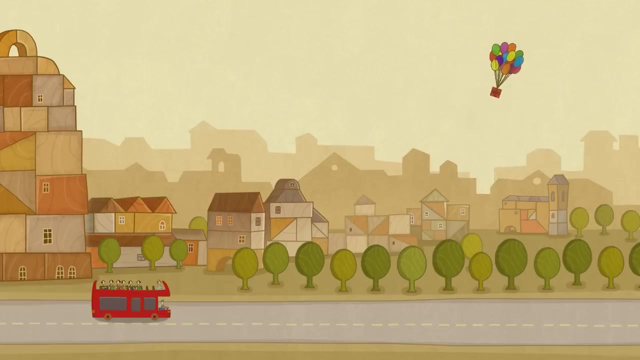 And he will miss the bus When he comes home. he does not waste a single penny. He drives around the bus every day. He drives around the bus every day. They are flying away, Prabhu, And here is an inter-city bus. 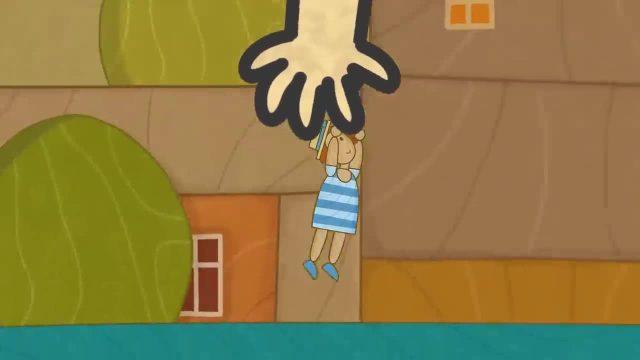 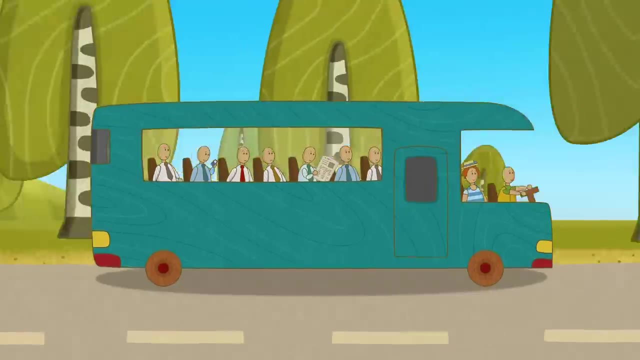 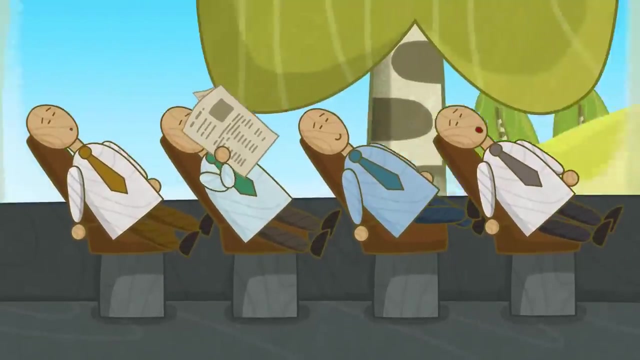 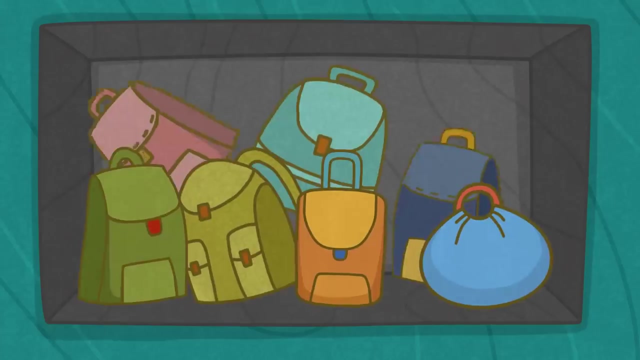 It carries passengers to other cities and even to other countries. An inter-city bus is on the road day and night. That's why there are special seats so that the passengers can sleep. Also a toilet, a TV, a fridge and plenty of room for luggage. 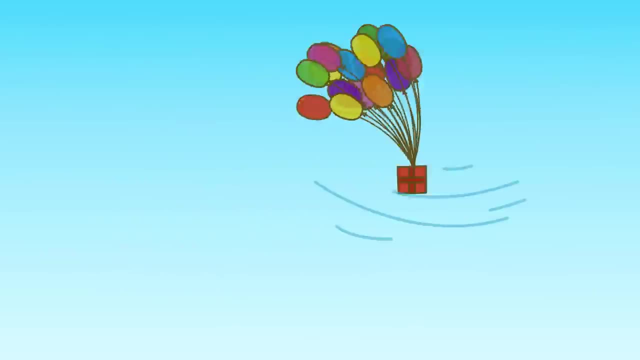 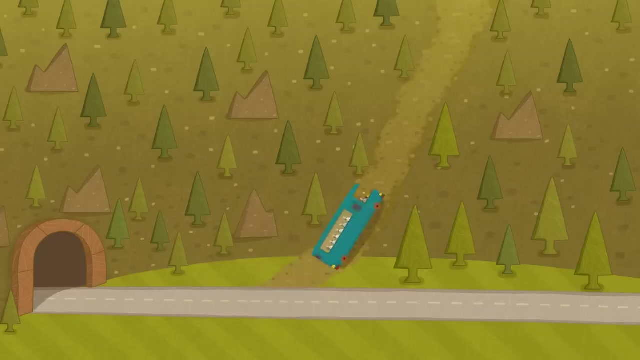 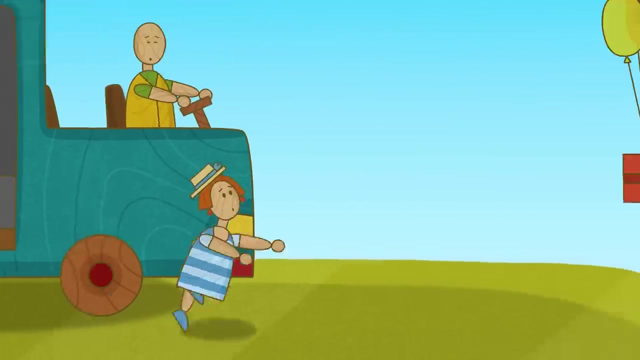 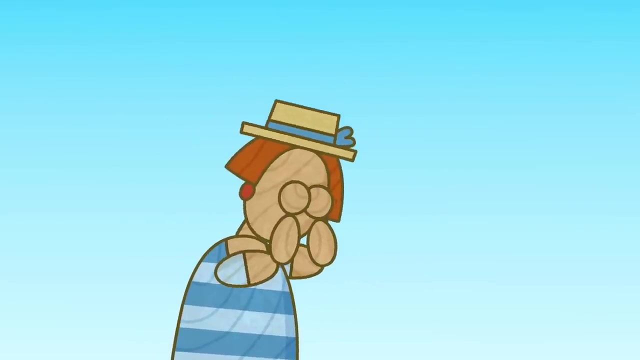 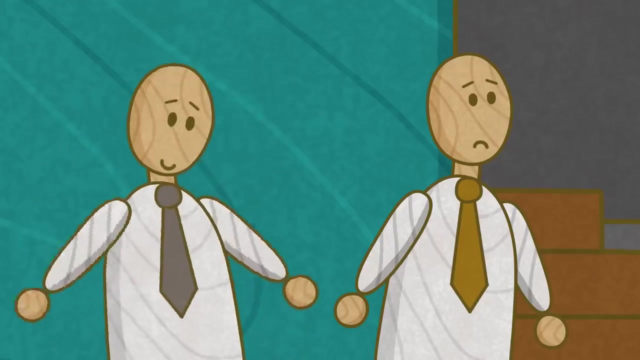 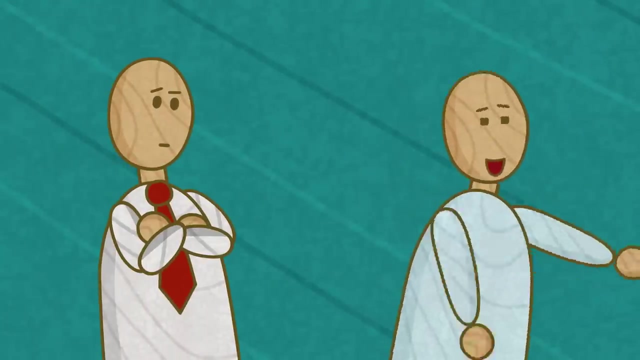 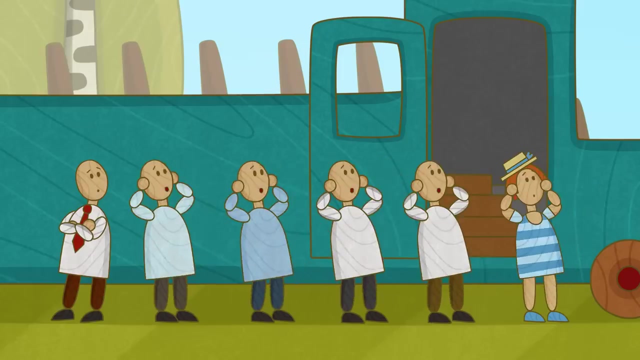 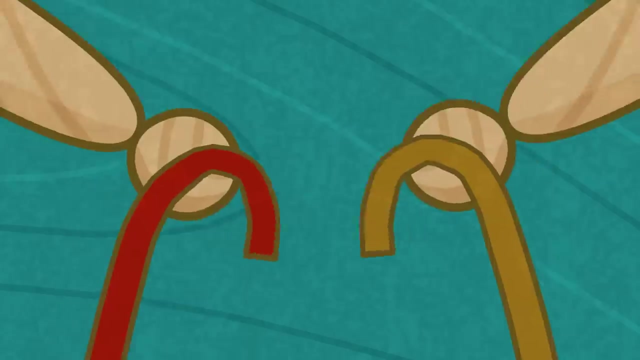 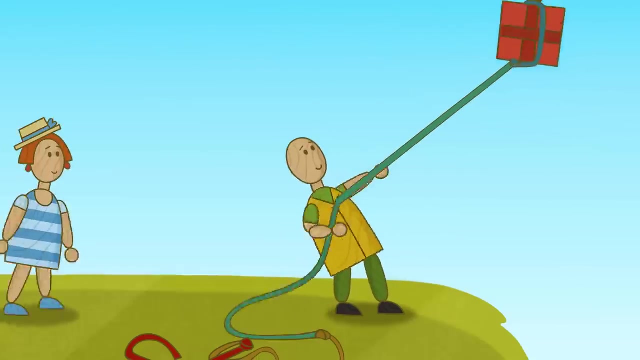 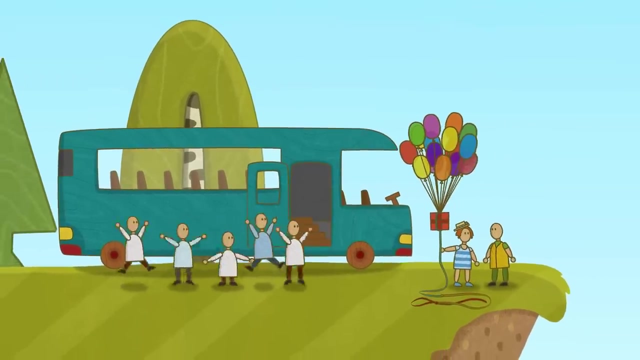 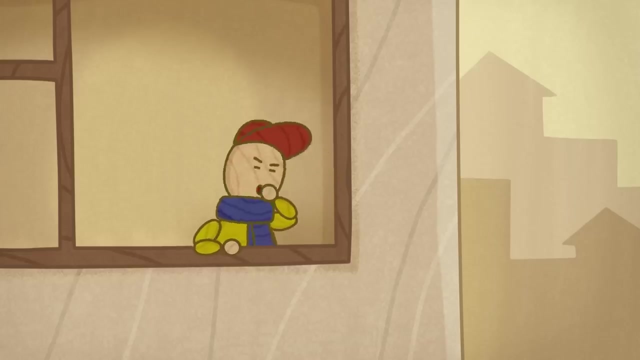 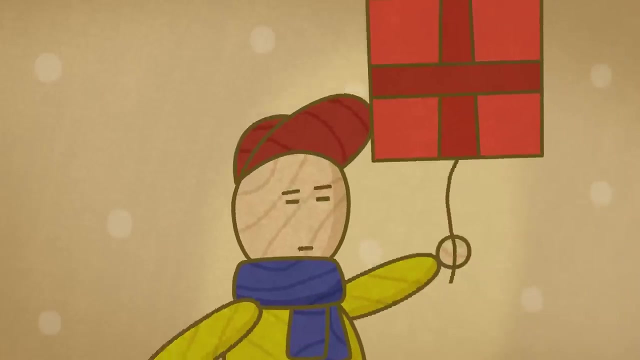 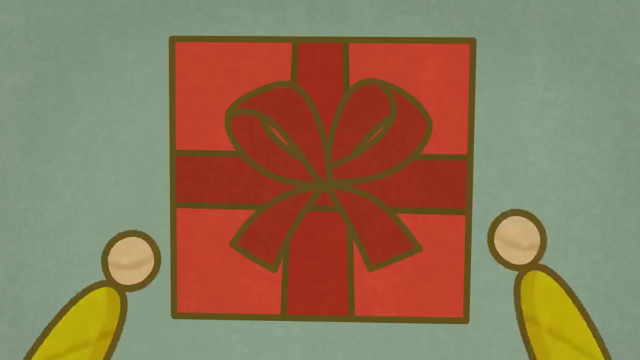 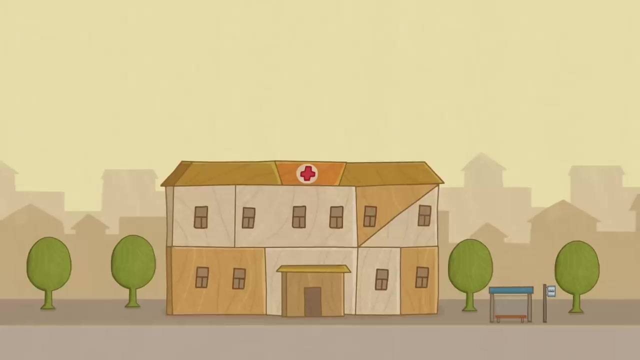 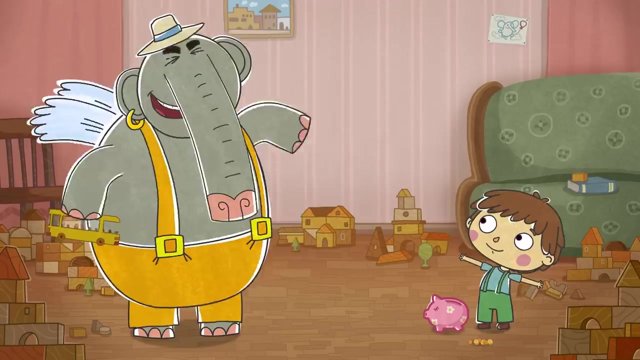 Even normal passengers can sleep here. Poo, Poo, Pu, Pu Pu. Oh Hey, Haha, Prabhu, let me take you for a bus ride. Great, it's been a while since I got on the bus.